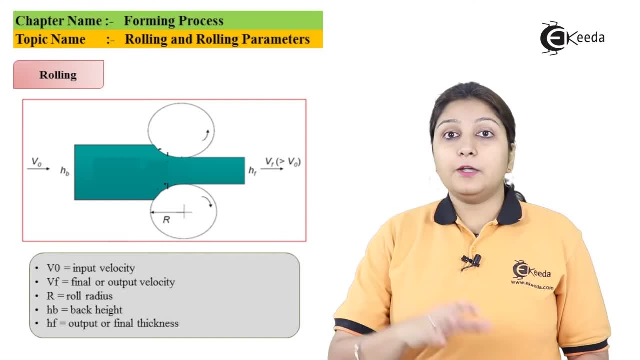 due to friction, your material is pulled and it goes to the other side, like from one side to the other side, and the thickness of the material is reducing. now how it is done. it can be done through cold rolling as well as hot rolling process, but the grain switches inside the material. 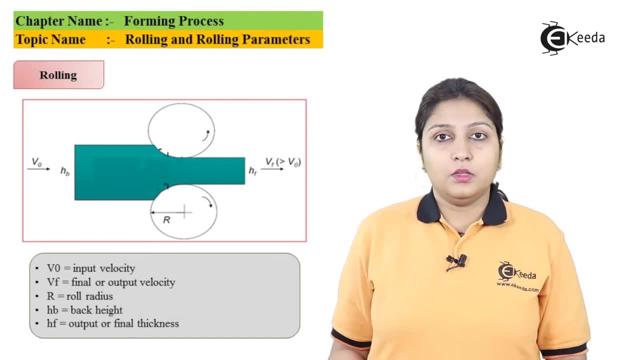 bends and it gets crushed and it gets joined. so in this way thicker part can be rolled to form thinner parts. so the nomenclatures we can see in this diagram is your input, velocity, roll radius and your height, which is given, height, which is more and less, and the entrance is more and the 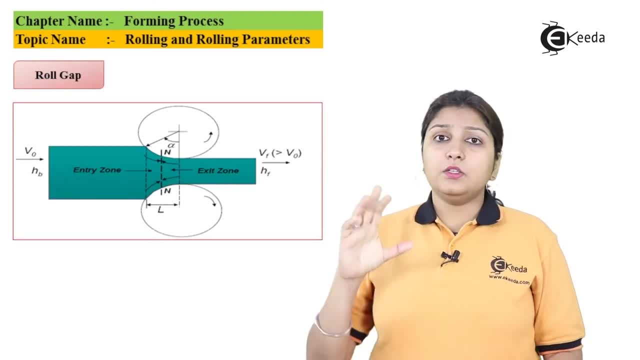 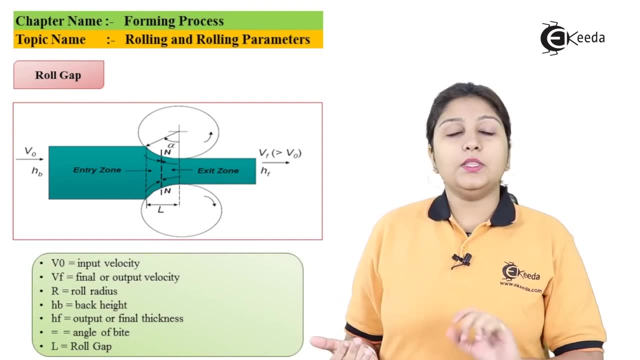 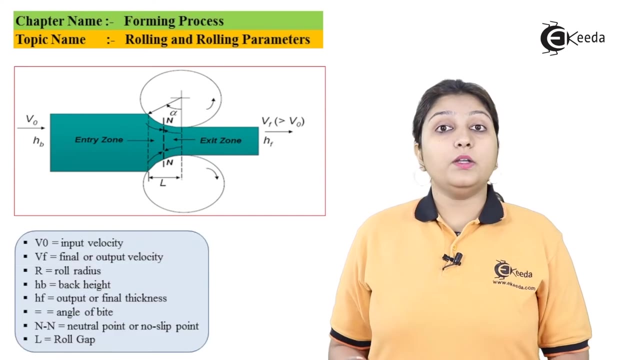 end is less. so i'll talk about roll gaps. can you see? the two rollers and the object is passing to is an exit zone, so between that there can be a roll gap which is formed. so now in this diagram, i'll just talk about the velocity. what is velocity, basically? if i say you a basic example, when your 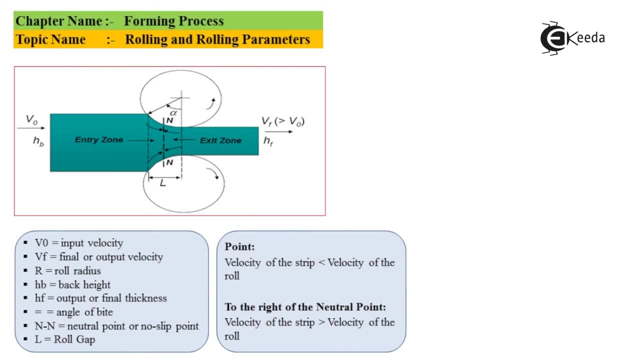 roller is coming and your object is coming between the rollers. what happens? the object passes through the rollers. so the entrance velocity would always be more and the inlet velocity would be less. so velocity of the roll plays a major part. your entrance velocity, like the entrance, will where. 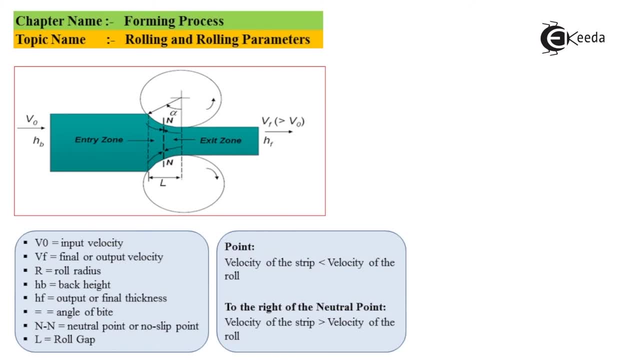 your exact role is coming would be always less than your roll velocity. and i'll talk about the exit. your exit velocity would be always more than your roll velocity. so this phenomena is always used in rolling because of the friction, because of the pulling of the roll. it is very 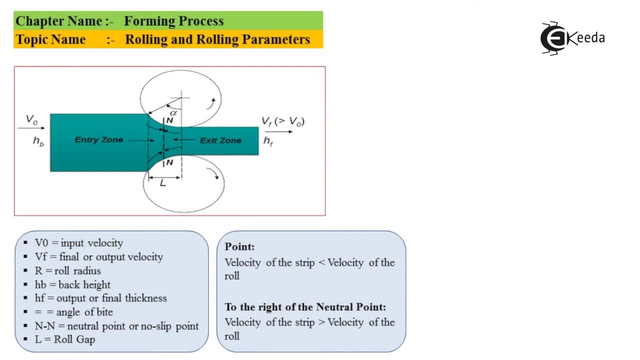 simple: whenever an object is pushed between the rolls it is going out outside, it will go at a very high pace rather than coming. coming would be very difficult, as it has to get squeezed between the rollers. so hence it is proved that outside velocity is always more so in this slide. 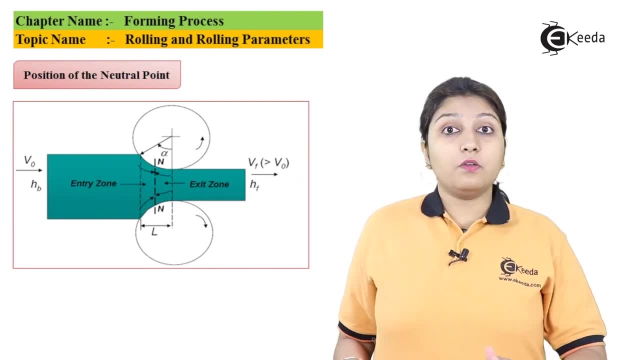 i'll just talk about. one of the major parameter is position of the neutral axis, which is between your entry and the exit zone when your rolling is done completely, when the last part of your object or your material is passing through your neutral axis, your roller skids so it